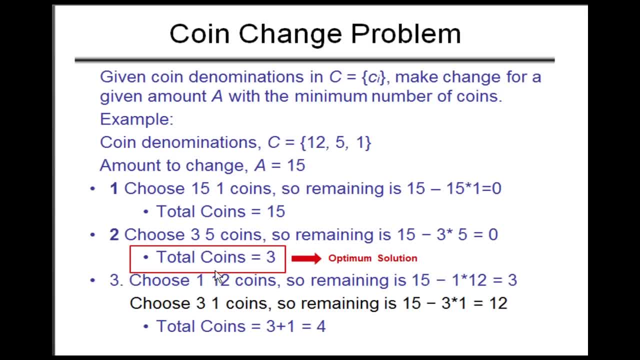 Way, or you could use one, You could use twelve dollar coins and you could use three one dollar coins And you could make, and with all together, four coins. you can make a fifteen dollar coin. now, still, that would take four coins And this would take three coins. so this is the optimal solution in this case. now Let's look at the algorithm. 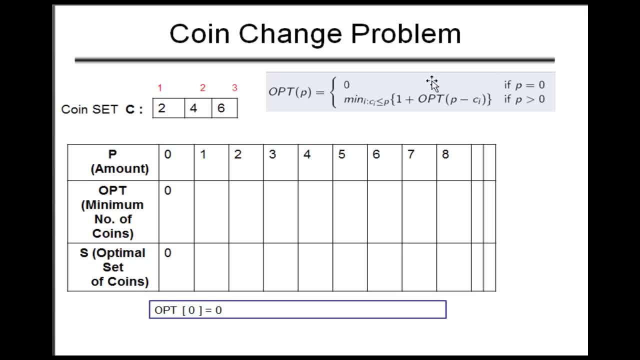 Yeah, so the algorithm is this is that when P equals zero, that time it's zero. the Optimum solution, that is, the minimum number of coins required is zero, But otherwise, when P is greater than zero, that time you take use this formula. now Let's look at the simulation. you'll understand what this formula means in a bit. 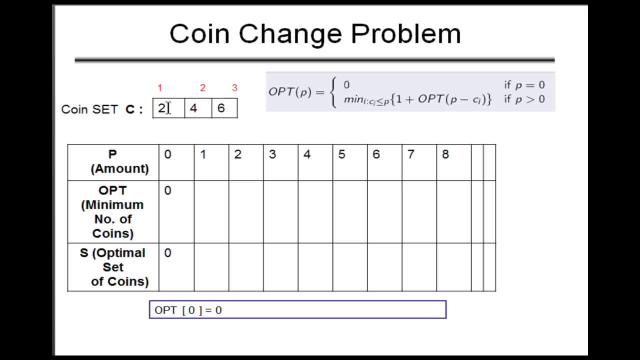 Okay, so for these are the set of coins given to do. you have two dollars, you have four dollars and you have six dollars. Now you have to make up to eight dollars. you have to make the change for eight dollars. So let's look at the simulation first. 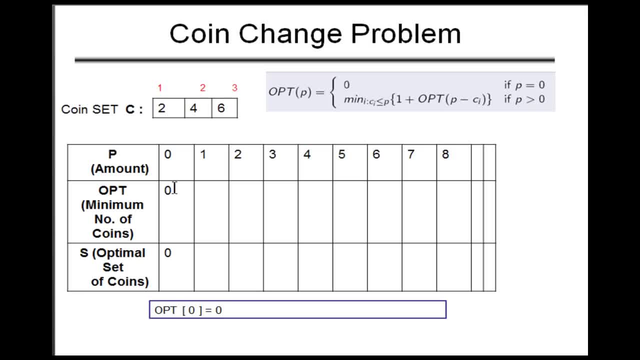 Let's look at four, four, four, the. Let's look at the table. There is base case, given, that is, when P equals zero. the optimum P, optimal solution is zero. the minimum number of coins required is zero. this is the base case, and For one also it will be zero because the set of coins start from two and then four and then six. so also for one. 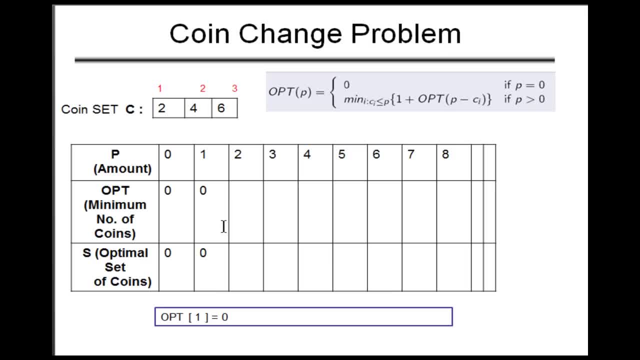 You have zero because you have no change for one dollar. you have to just, you have to just get two dollars and $1 you'll get back as a change from the shopkeeper. but for You don't have any one dollar coin on its own for $2. You can just give one coin and you could just give. 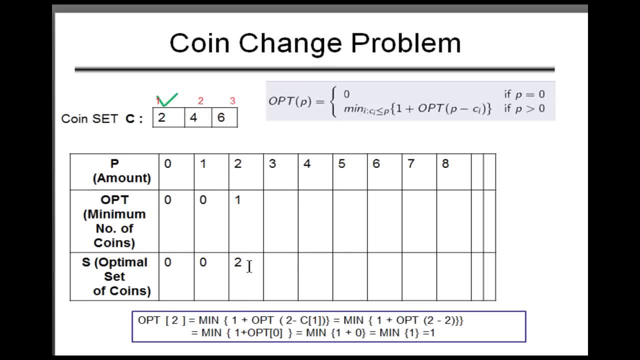 Two. you can just give one coin. the minimum number of coins is one and you have to give the two dollar coin. How did we compute this? Let's look at the simulation here. opt, P, opt to is. We get it by using this formula: mean of one plus opt, P minus CI, P is two here, because we have 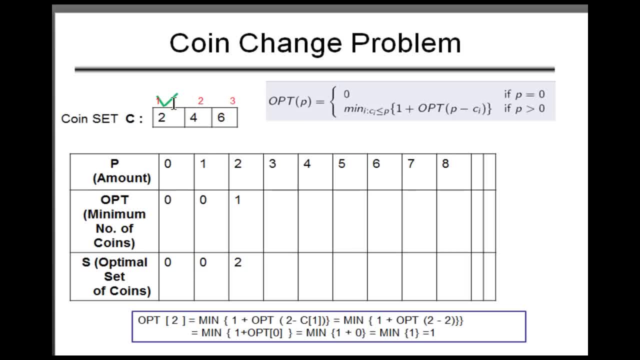 Gone till two only. so two Minus CI, CI is C: 1 because we have just reached till this. when we reach for that time, we can use two and four. when We reach six, that we can use all three sets of coins now, since we have reached just the first set of coins. 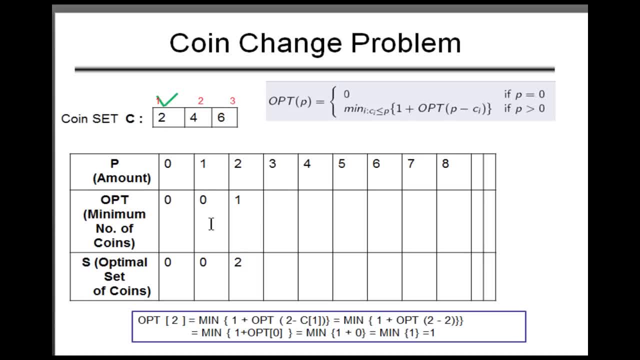 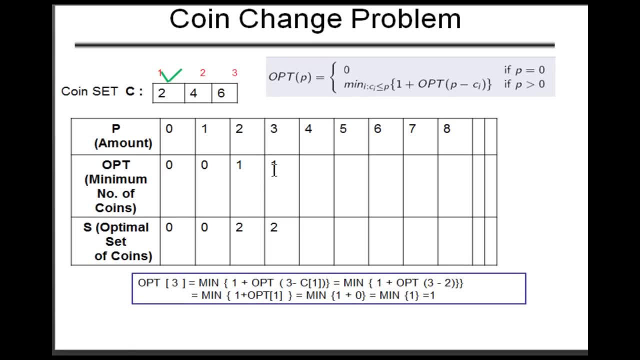 So we just used to now and then for. so this is for two, and then let's compute the one for opt three. For opt three it will be like this: For opt three is mean equal mean of one plus opt three minus C one Now mean the mean thingy is not being used right now. 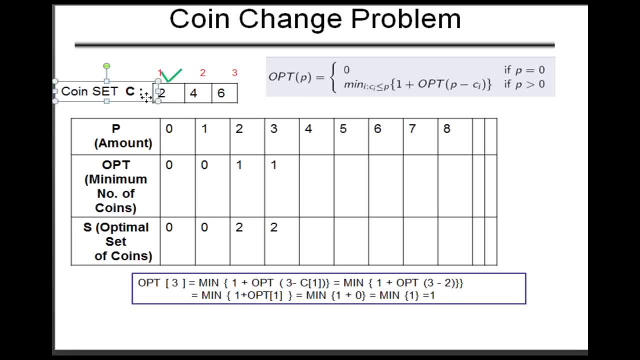 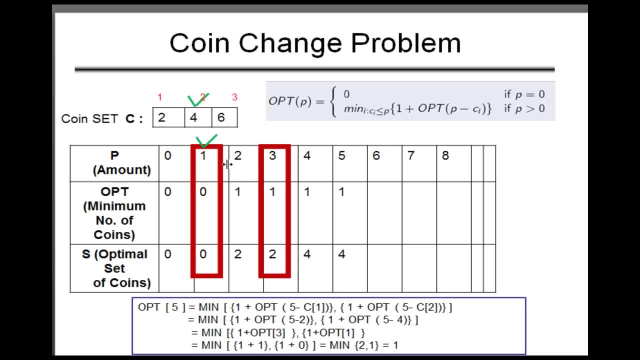 It will come to use when we, when we go to the other sets of coins, since we are just using one set of coin. That's why, oh, Since we're just using one set of coin, That's why it's like this. all right, so for Opt three, it will be one plus opt. 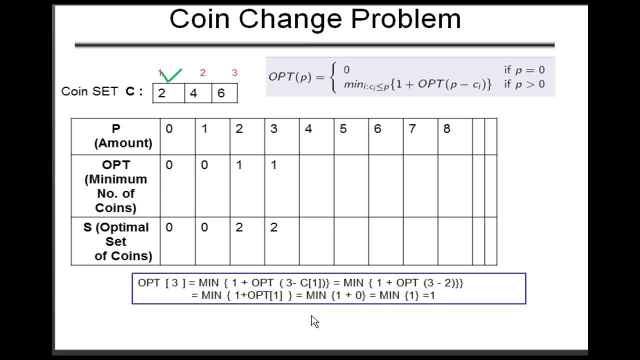 Yeah, so it will be one plus opt five. yeah, three minus C one, three minus C one, three minus two, so three minus two, one plus opt, three minus two, which is one plus opt of one and Opt of one. we know that opt of one is zero, so one plus zero is one. 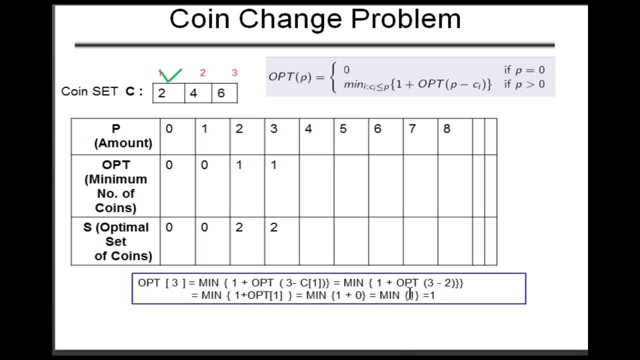 So the minimum, there's just one number. that's why there's just one will be the answer. So opt is one, and for this we just need two dollar, two dollar coins, Because we don't have any change for one dollar coin, So we just have one change for it. and then you just have to manage and tell the shopkeeper that well, you want three. 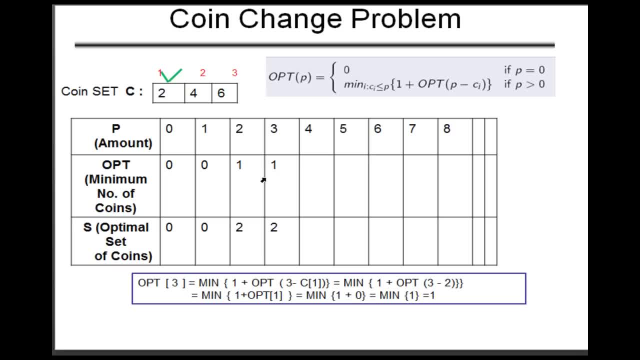 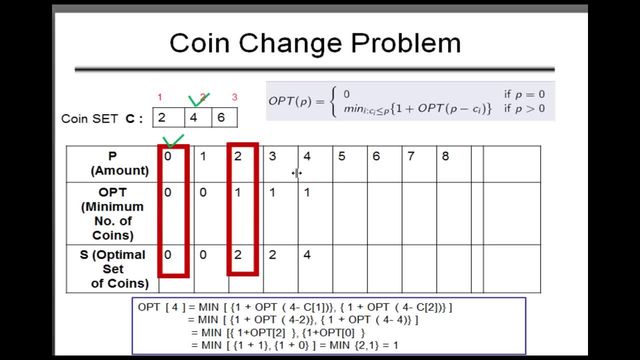 dollars. Well, I just have two dollars coins. I can't give you the other one, so just keep just bear with me for the change. anyway, for the fourth one, when you have four, you can like in your mind you can think that, yeah, you can just take two, two dollar coins, or you can. 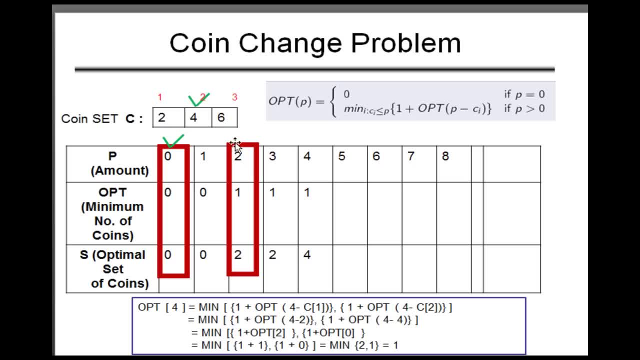 just take one four dollar coin, which you already have, so we could just use this one because we're using for the. we're trying to minimize the number of changes. that's why we're gonna use this one. so how did we compute this mean of one opt? 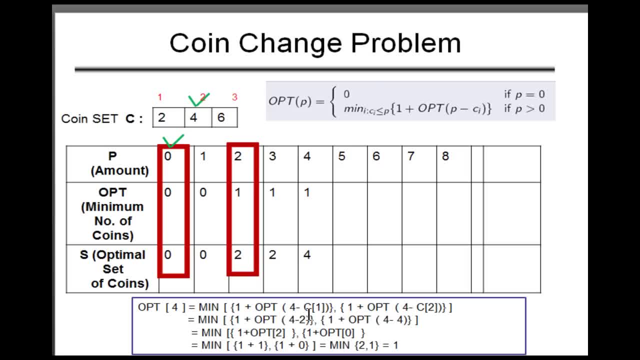 is not for us, up is not for so. P minus C 1 and the comma, we have 1 plus. opt for minus P minus C 2, because we have reached to 4, so we can use these two denominations, these two sets, these two coins set together: P 1, I mean C 1 and C. 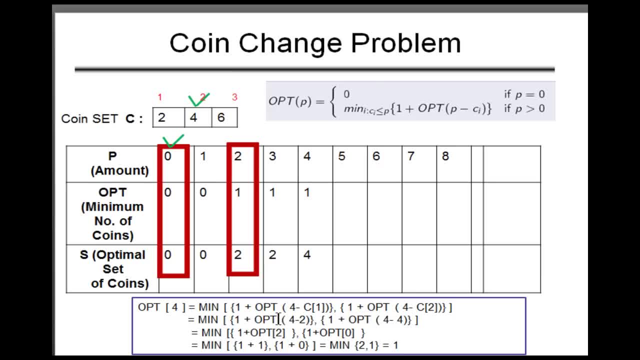 2. so we just drive for C 1 and we just drive for C 2, and then we compute so 1 plus opt for minus 2 and 1 plus of 4 minus 4, and then 1 plus opt 2 is opt 2. 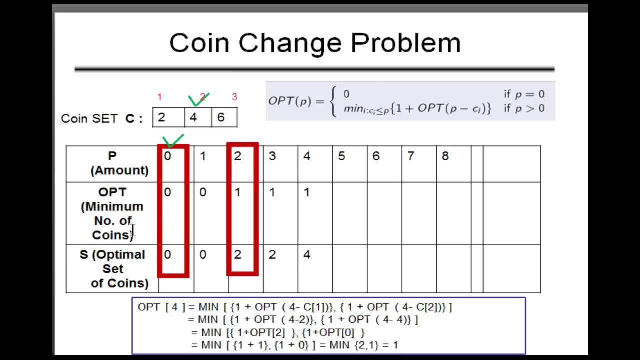 is 1 and 1 plus opt 2. opt 0 is 0, so 1 plus opt 2 is 1, so 1 plus 1 and 1 plus 0. so the minimum of 2 and 1 is 1. so the opt for 4 is 1. alright, and the optimal set of coins is 4, because, since we are just 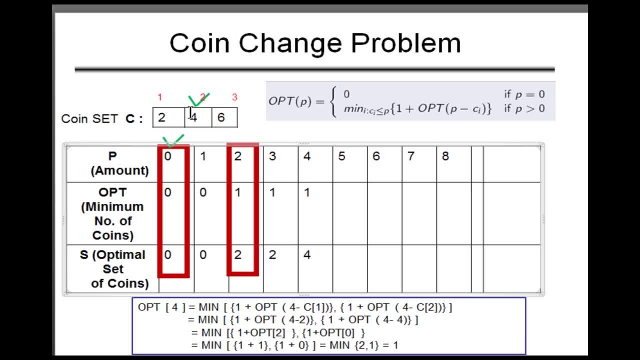 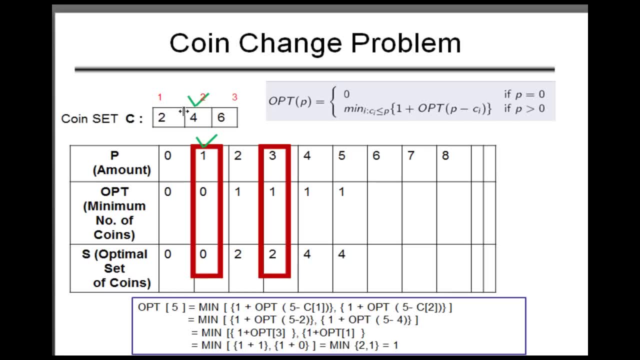 taking 1 coin. so 4 is the optimal solution. 4 is the coin that we are taking, alright for 5. 5 also, we do the same thing. since we just reached 2 and 4, we can't use the 6th c3 yet. 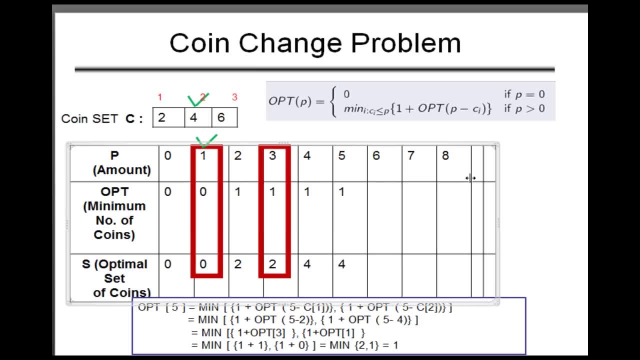 because we can only use it after we reach 6, the 6th table. alright, ok, so 1 plus opt, 5 minus c1, and then 1 plus opt, 5 minus c2. so 5 minus c1 is what? what is c1? c1 is 2, so 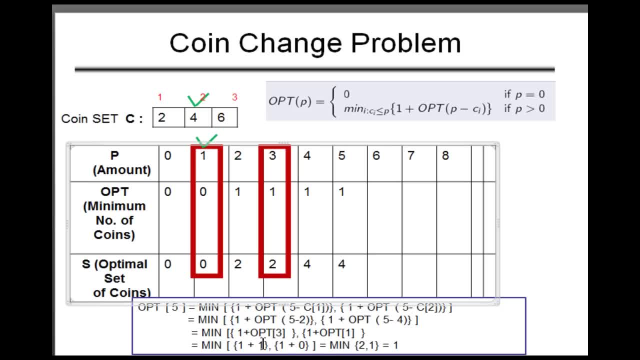 5 minus 2 and c2 is 4, so 5 minus 4, so 1 plus opt 3. opt 3 is 4, so 5 plus opt 3 is 4, so 5 plus opt 3 is 1. so we use this one opt 3, 1 and then 1 plus opt 1. opt 1 is 0, so 1 plus. 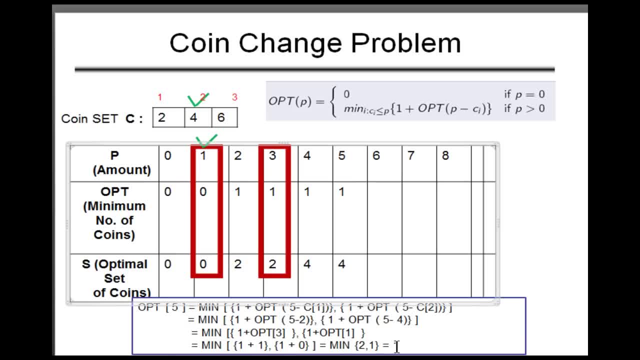 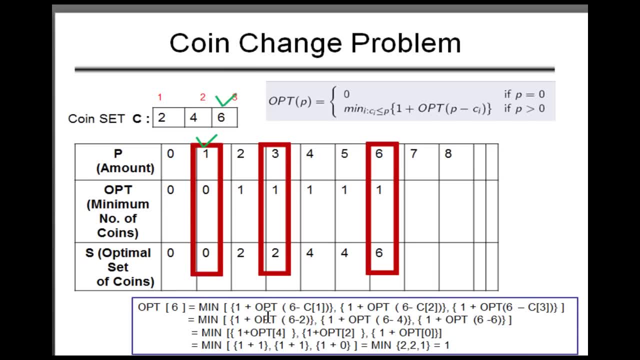 1 and 1 plus 0. so again, the minimum between these 2 numbers is 1. alright for 6. now that we have reached 6, lets look at the algorithm now. 1 plus opt c1, 6 minus c1, that means P. 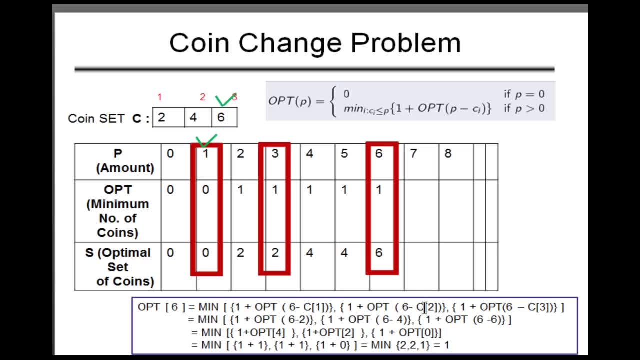 minus ci, so 6 minus c1, and the one plus opt, 6 minus c2, and 1 plus opt, 6 minus c3. so we do the same thing for Rotaryjs grapes. same thing: 1 plus opt, 6 minus 2, c1 is what you call 2 and c2 is 4 and c3 is 6, and then 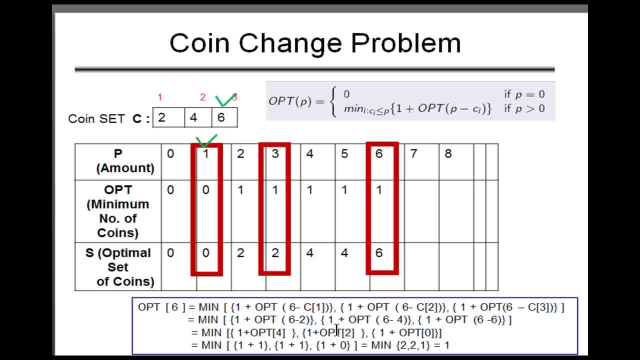 1 plus opt 4. we look at the table: opt 4 is 1, 1 plus opt 2. opt 2 is 1 again and opt 0 is 0. so we try to find the minimum between 2, 2 and 1, which is 1. so we just use 1 coin. 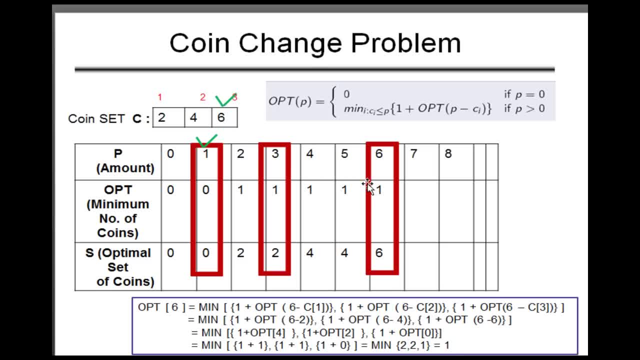 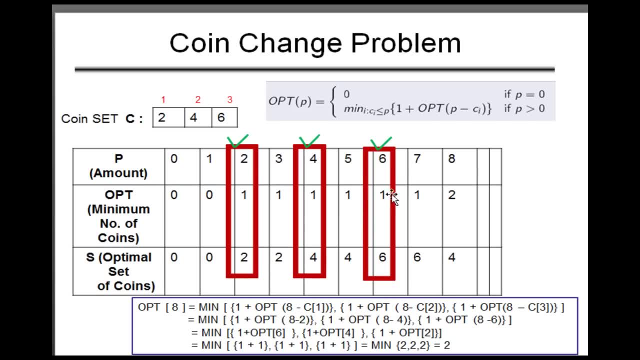 for this. we just give the 6 dollar coin to the shopkeeper, so that's why we just use one denomination. like i said, we're trying to minimize the number of denominations. all right, for the seventh one, the seventh coin, we do the same thing again. well, the tutorials just. 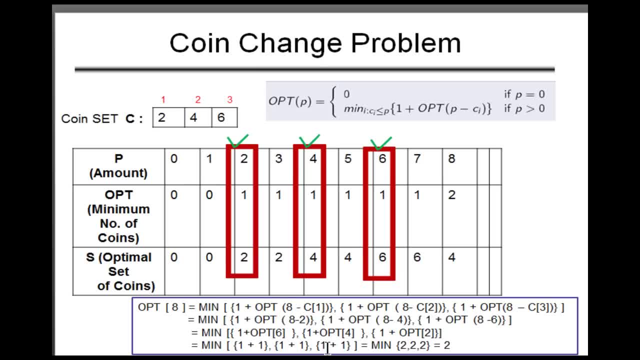 goes this way. i mean now, i think, after showing you few examples, you can do the compute. the rest, let's look at the seventh one. uh, seventh one is all right. let's look at the eighth one instead, because seventh one is quite easy. let's look at the eighth one, the last one. 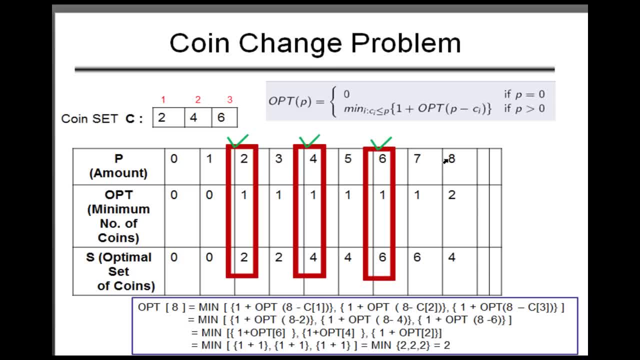 what we have to do with the last when you reach the last coin that we're trying to change. uh two find changes of: so 8 minus c1, 8 minus c2, 8 minus c3, 1 plus opt. 8 minus 2 c1 is 2 c2. 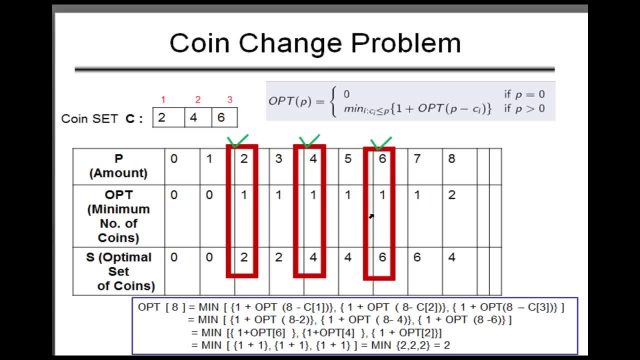 is 4 and c3 is 6, so opt 6 is 1, opt 4 is 1 and opt 2 is also 1, so 1 plus 1, 1 plus 1, 1 plus 1, so the minimum for these three is just 2 itself. now 8 can be broken down into two. 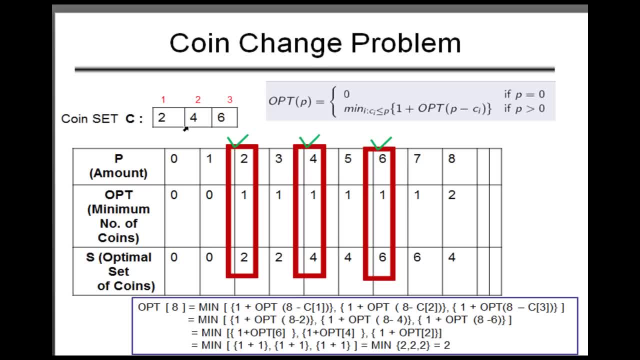 two denominations. by using 6 plus 2, 8 is 6, 7, 6 plus 2 is 8 or 4 plus 4, we can just use two four dollar coins, or we can just use one two dollar coin and one six dollar coin. does not matter, you can use any. you can use any solution because, since 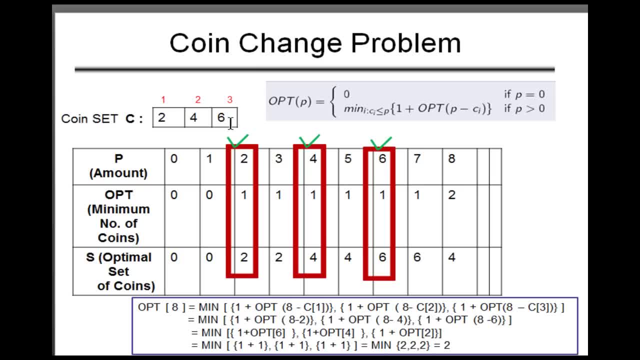 both of these solutions will give you two, two, two coins. i mean just two denominations, the two optimal set of coins. you can just choose any for this. for this example, we have just chosen two, four dollar coins. all right, so this is was. this was basically the whole. 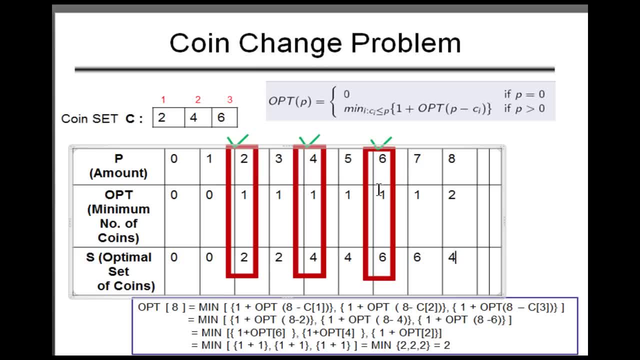 tutorial. i think this was, like i said, the easiest of all the dynamic programming algorithms. i hope you understood the explanation and please feel free to like and subscribe, and well, good luck.